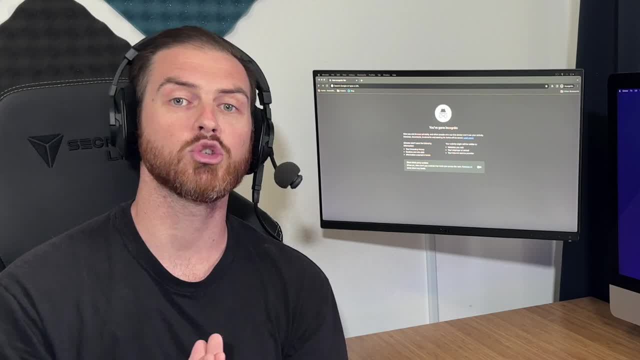 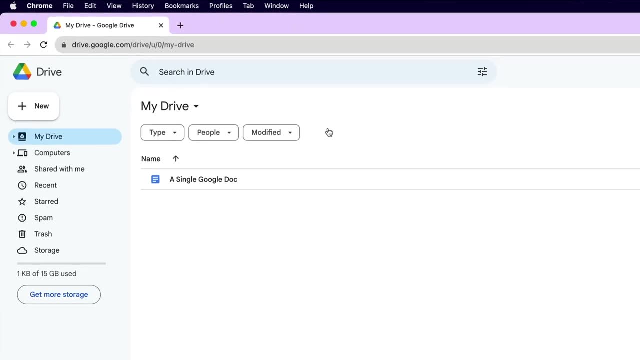 internet like normal. Everything that you do will be cleared as soon as you end your incognito session. So how do you end the session? Just close the window. It is that simple. You are now out of incognito mode. Now there are a few important things to note when using. 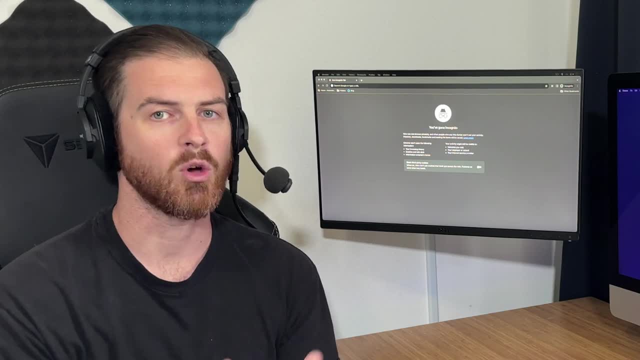 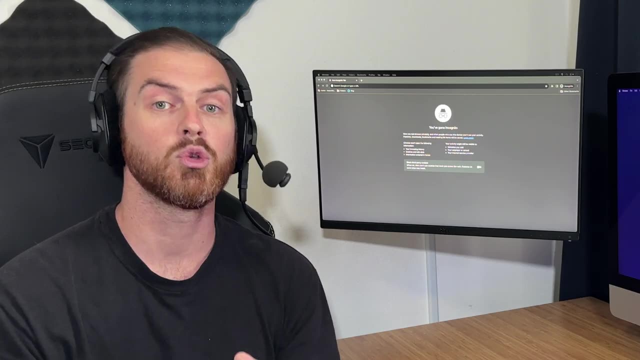 incognito mode. First of all, you can still browse normally while browsing in incognito, So you can have your incognito window up, and then you can have a normal browsing window at the same time, So you can use both accounts simultaneously, one in an incognito window. 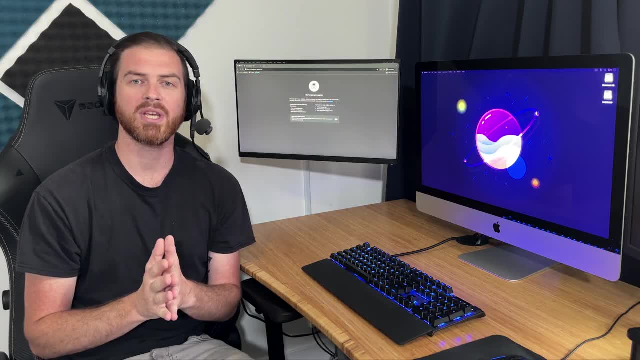 and one in a normal browsing window. Also, although your browsing history and searches won't be saved while you're in incognito mode, you'll still see saved searches and browsing history from your normal browser window, So you can use both accounts simultaneously. 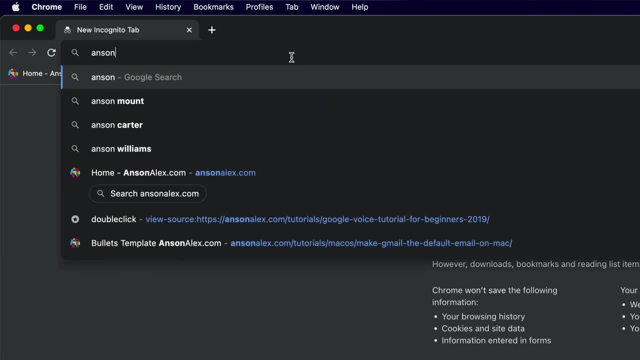 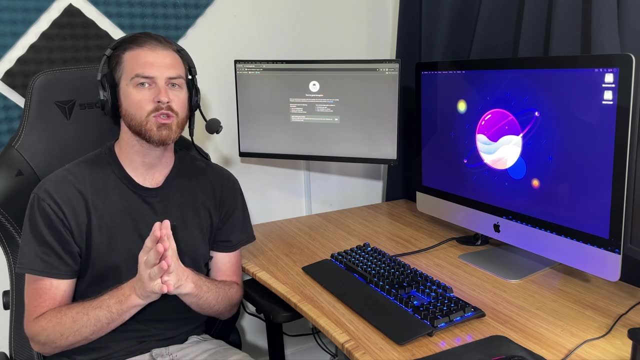 So if you're in incognito and you go up to the address bar and you see some websites auto filling, don't worry, Those are from your normal browsing sessions. If you want to clear your browsing history from your normal sessions, you can always go up to the three little dots. 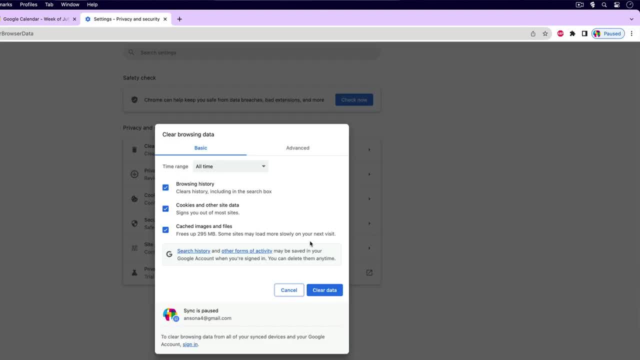 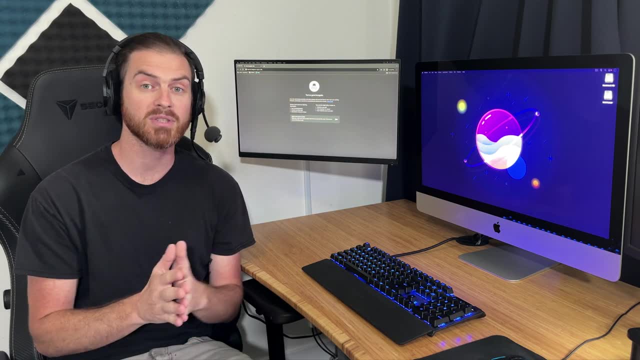 go to more tools and then clear browsing history. In regards to privacy, incognito mode does a great job of making sure that there isn't any information stored on your computer from your browsing session. However, when you're browsing the internet, your IP address can still be tracked. 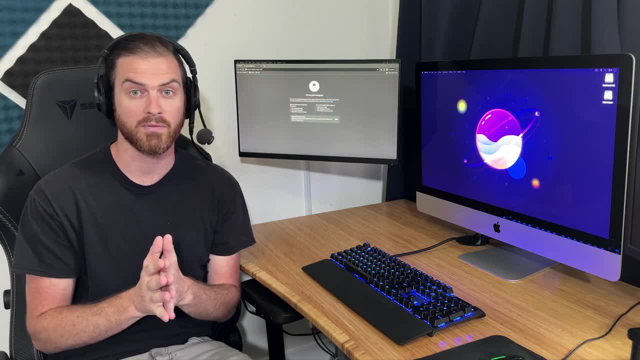 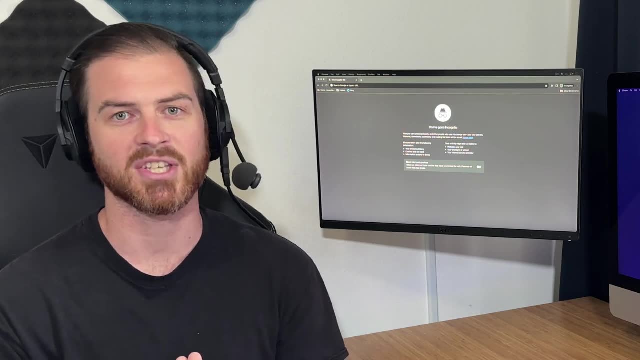 And incognito doesn't block that. You would need a proxy server for that. For most users, this isn't an issue, but I just want to give you all of the details so that you know what incognito does and doesn't do. One last thing to note is that, because you're not saving cookies and site data when using incognito. if you're logging into accounts that require two factor authentication- so accounts that require either a text or an email confirmation- you will have to go through that two factor authentication every single time you log in. 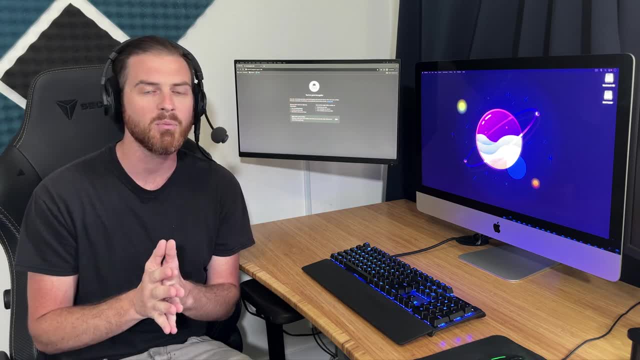 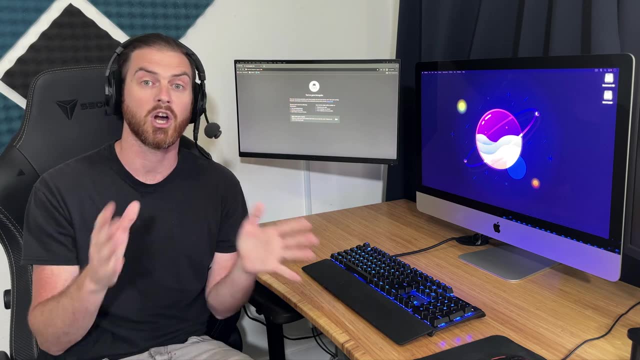 to incognito mode. This isn't really a limitation of incognito mode. It's just a side effect of private browsing when you're not storing that information. So do be aware of that if you are going to be using incognito mode to log into multiple accounts. So there you have it That. 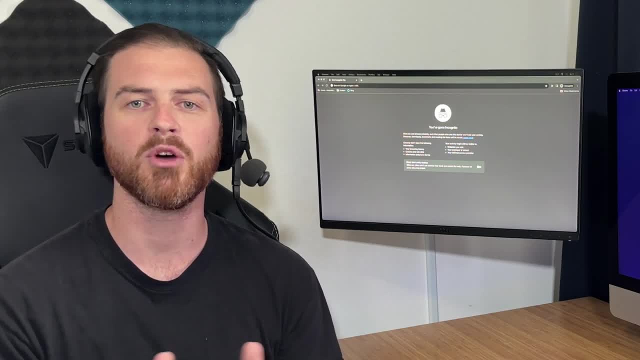 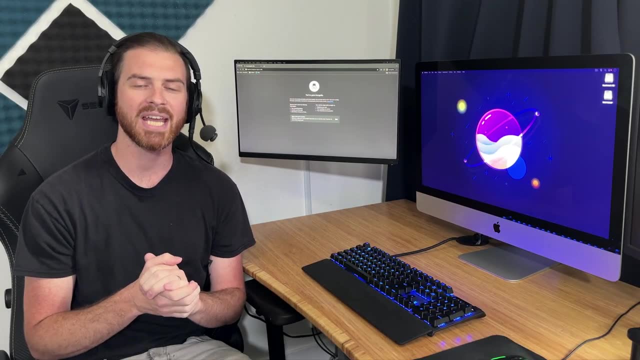 is pretty much everything that you need to know about using incognito mode in Google Chrome and private browsing on the internet in general. I hope that you found this video helpful. If you did, I would really appreciate a thumbs up here on YouTube And if you want to see more guides.